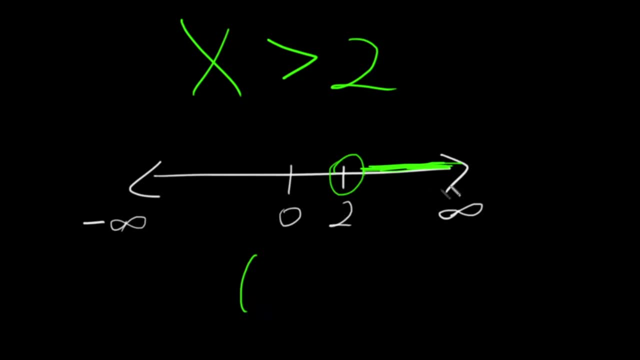 to put the numbers from smallest to largest, In this case left to right. The farthest to the left we get is 2.. We'll start with 2.. We always put a comma between the numbers, And then we go all the way to the right without stopping. So we'll go all the way up to infinity, And then we 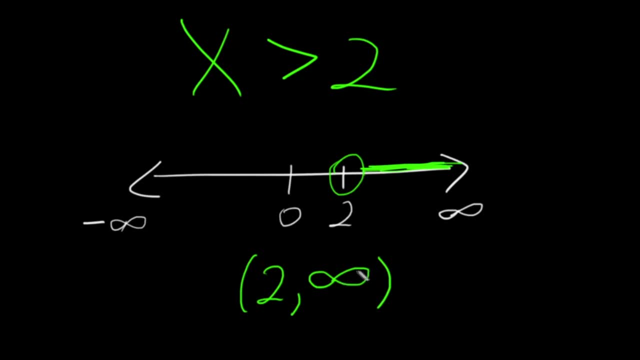 always use parentheses with infinity, regardless if it's positive or negative, since it's a concept and not an actual number. Now what if our inequality was x is greater than or equal to 5?? Like before, we'll use a number line. If 0 is here, 5 is going to be to the right over here. 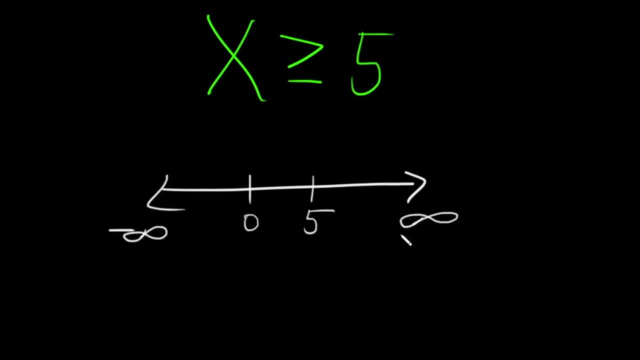 Negative infinity to the far left and positive infinity to the right. In this inequality, we're greater than or equal to 5.. This time it's not going to be an open circle, but a closed circle at 5 to indicate that we're. 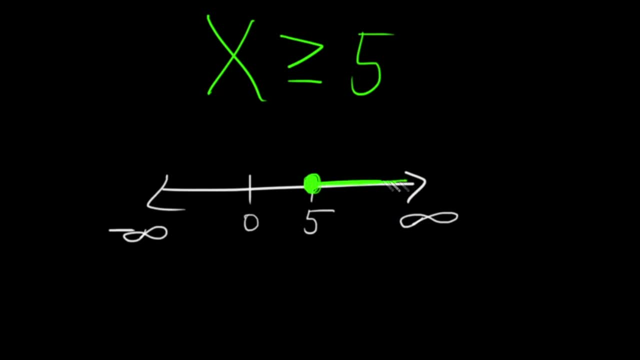 including the 5 here, And then we'll shade to the right, since x was greater than or equal to 5.. Using interval notation, we can list the numbers from left to right. The farthest to the left we get was 5.. So we can start with 5, comma and we go all the way up to infinity, But this time 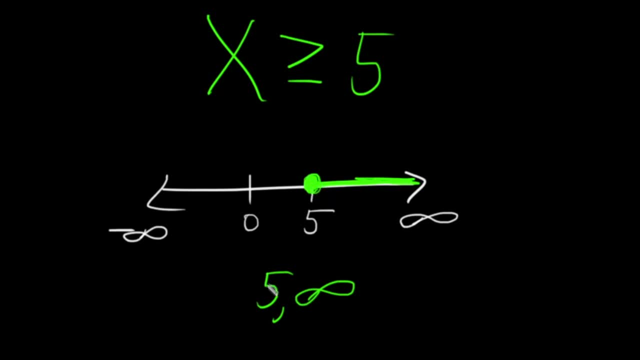 since we were greater than or equal to, that gave us a closed circle, And we're going to represent that with a bracket this time, to show it includes the 5.. And, like before, anytime there's infinity, we have to use a parenthesis, So anytime we have a less than or greater than sign. 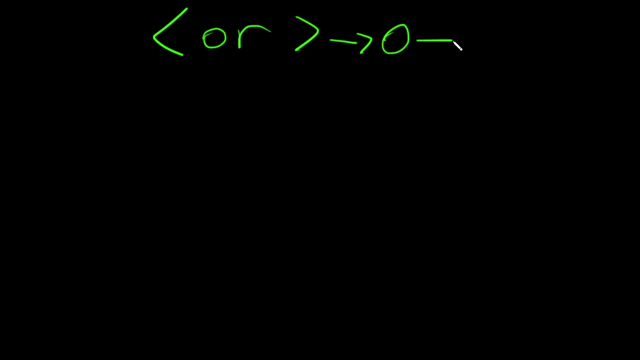 then on the number line we'll need to use an open circle And with interval notation that's going to need a parenthesis. On the other hand, if we have less than or equal to or greater than or equal to, then on the number line we're going to use a closed circle. 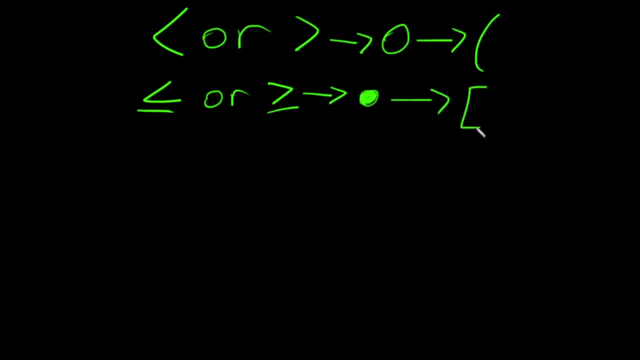 And with the interval notation, that's going to need a bracket. Finally, with positive or negative infinity, we're always going to be using a parenthesis. Let's look at another example. Say we have x is less than 1. We'll draw the number line. 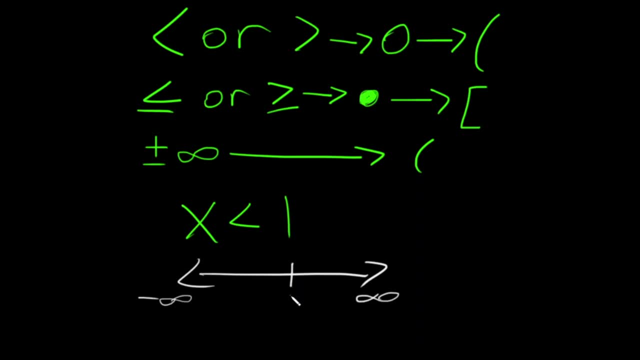 from negative infinity to infinity. Let's place 1 right here. x is just less than 1, not or equal to, which means we're going to have to use an open circle, since we're not including the 1.. And then for the shading we need to use the numbers less than 1,. 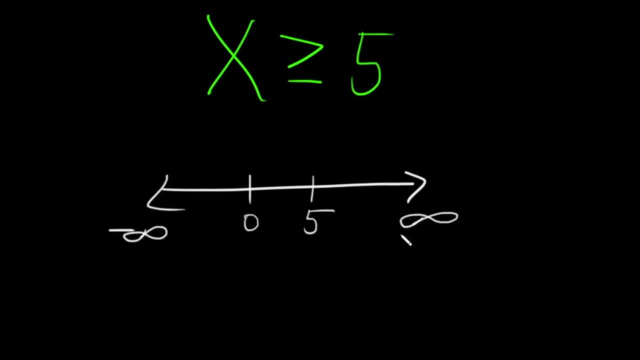 Negative infinity to the far left and positive infinity to the right. In this inequality, we're greater than or equal to 5.. This time it's not going to be an open circle, but a closed circle at 5 to indicate that we're. 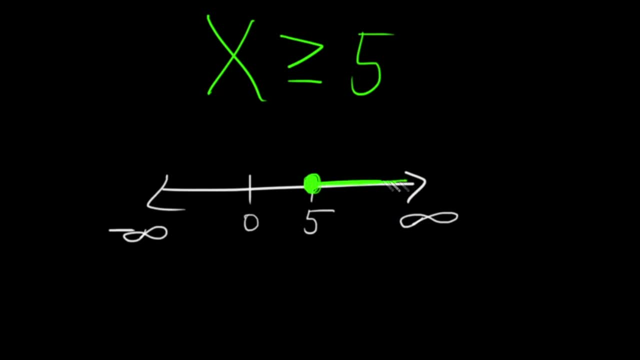 including the 5 here, And then we'll shade to the right, since x was greater than or equal to 5.. Using interval notation, we can list the numbers from left to right. The farthest to the left we get was 5.. So we can start with 5, comma and we go all the way up to infinity, But this time 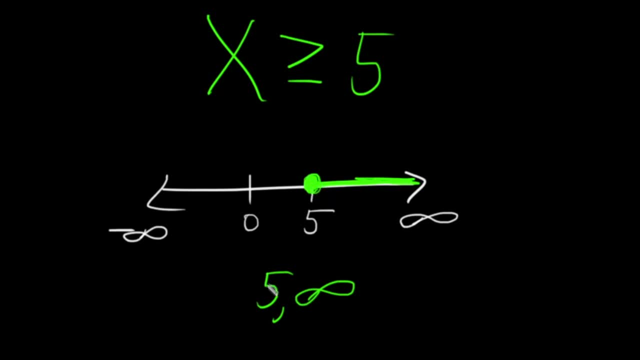 since we were greater than or equal to, that gave us a closed circle, And we're going to represent that with a bracket this time, to show it includes the 5.. And, like before, anytime there's infinity, we have to use a parenthesis, So anytime we have a less than or greater than sign. 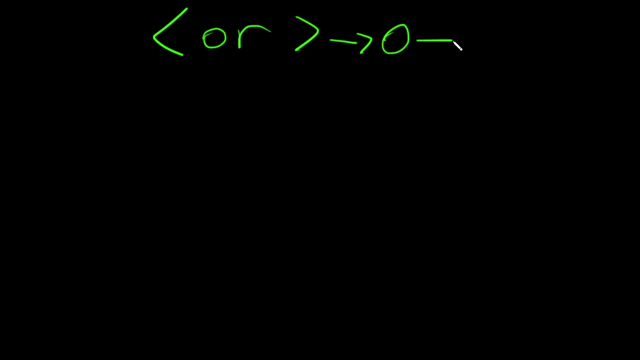 then on the number line we'll need to use an open circle And with interval notation that's going to need a parenthesis. On the other hand, if we have less than or equal to or greater than or equal to, then on the number line we're going to use a closed circle. 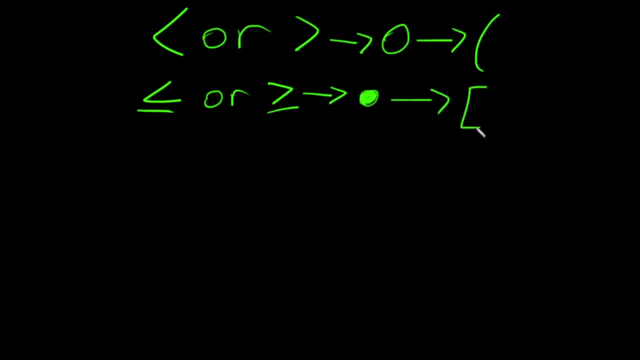 And with the interval notation, that's going to need a bracket. Finally, with positive or negative infinity, we're always going to be using a parenthesis. Let's look at another example. Say we have x is less than 1. We'll draw the number line. 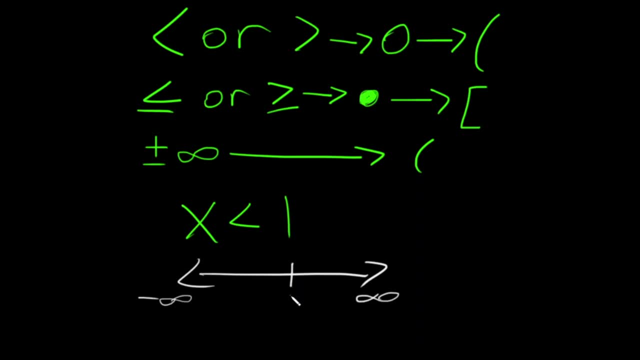 from negative infinity to infinity. Let's place 1 right here. x is just less than 1, not or equal to, which means we're going to have to use an open circle, since we're not including the 1.. And then for the shading we need to use the numbers less than 1,. 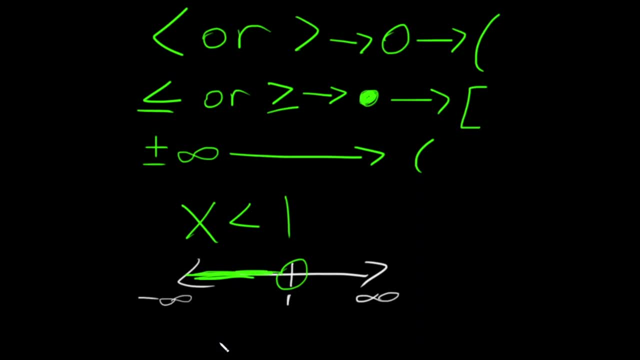 which would be going to the left. on the number line, Using interval notation, we always go from the smallest number to the largest or left to right. So the farthest to the left we go is negative infinity And, like we saw, positive or negative infinity requires a parenthesis. 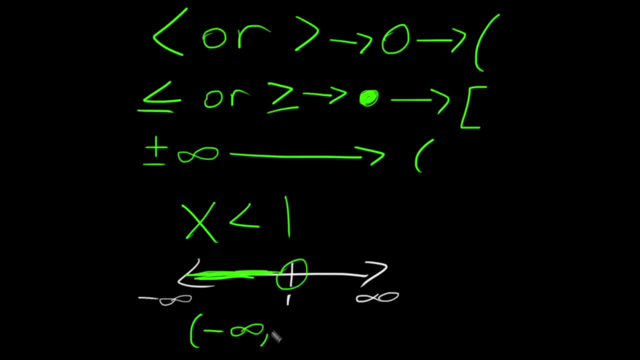 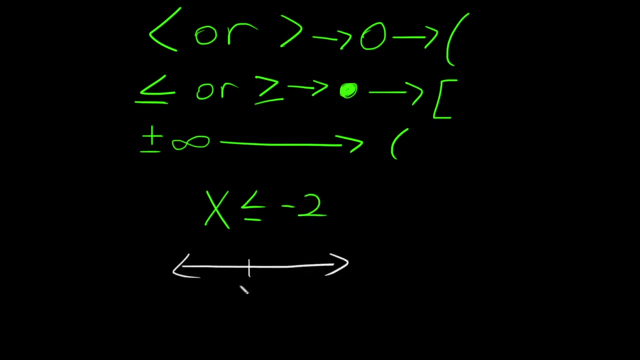 So we're going to open parenthesis, negative infinity comma, and then we go all the way up to 1 and open circle because we're not including, therefore close with parenthesis. Now, if we have x is less than or equal to negative 2, we have our number line negative 2 over here. 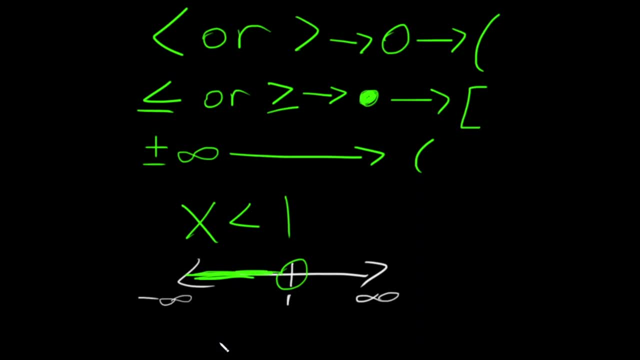 which would be going to the left. on the number line, Using interval notation, we always go from the smallest number to the largest or left to right. So the farthest to the left we go is negative infinity And, like we saw, positive or negative infinity requires a parenthesis. 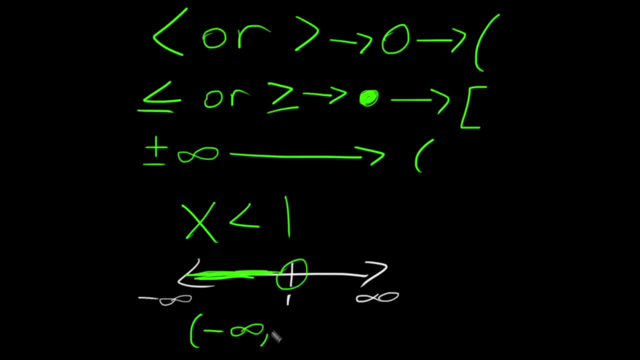 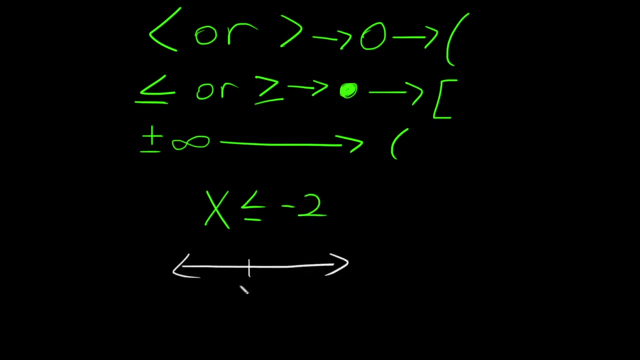 So we're going to open parenthesis, negative infinity comma, and then we go all the way up to 1 and open circle because we're not including, therefore close with parenthesis. Now, if we have x is less than or equal to negative 2, we have our number line negative 2 over here. 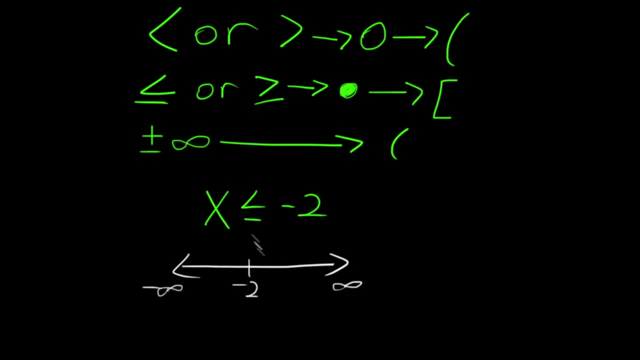 infinities. This time the x is less than or equal to, so we need to use a closed circle to show that we're including the negative 2. And we'll be shading to the left, since it was less than The leftmost amount is negative infinity comma and we're going up to negative 2. Infinities: 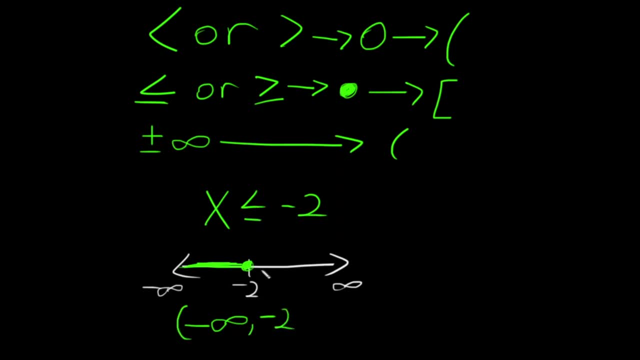 always have parentheses And this time, since we're less than or equal to and we have a closed circle, we're going to use a bracket. Now let's look at compound inequalities. Say, we have x, which is less than or equal to negative 3,, but less than 5.. If we're reading this, inequality left. 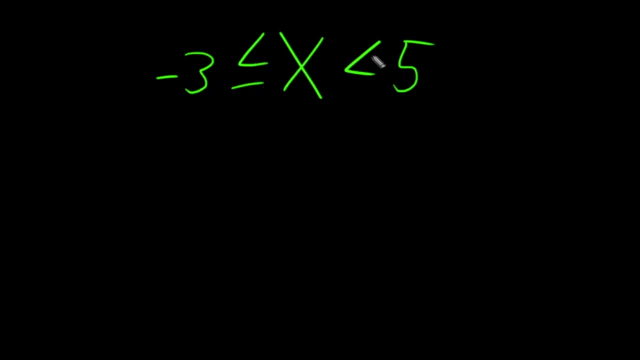 to right. it does say negative: 3 is less than or equal to x, which is less than 5.. But to keep it simple, we can read it starting with the x. In this case x would be greater than or equal to. 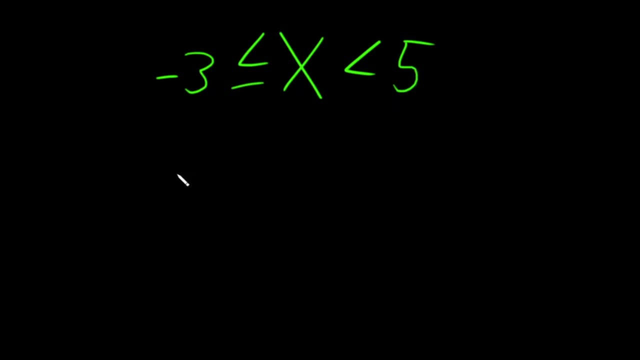 negative 3 and still less than 5.. First let's plot those two numbers on a number line. If negative 3 is over here, then 5 needs to be somewhere to the right over here. First let's do the circles and. 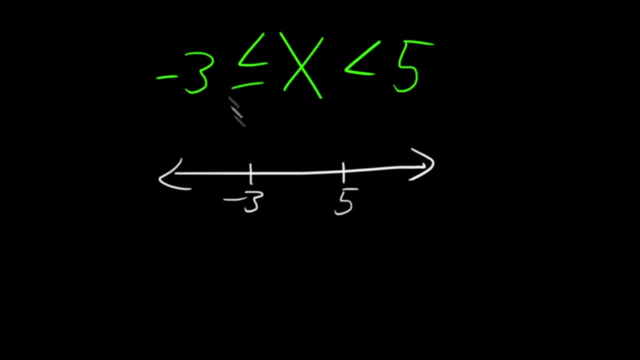 then we'll do the shading. x was greater than or equal to negative 3,, but less than 5.. If we're reading this, then x is greater than or equal to negative 3, so we're going to need a closed circle at negative 3.. On the other side, x is less than 5,, which does not include 5, so therefore we 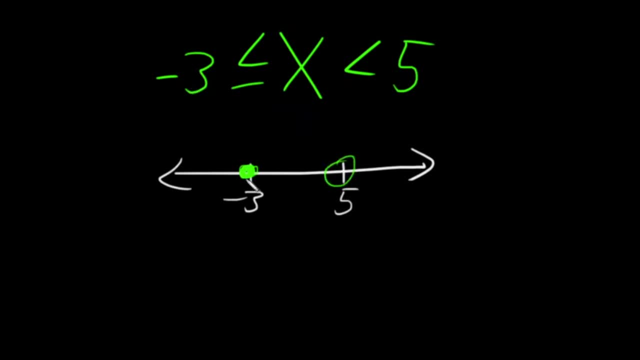 need an open circle. Since x is greater than or equal to the negative 3,, we need to shade to the right from negative 3.. And looking at the 5 side, x is less than 5, so we need to shade to the left. 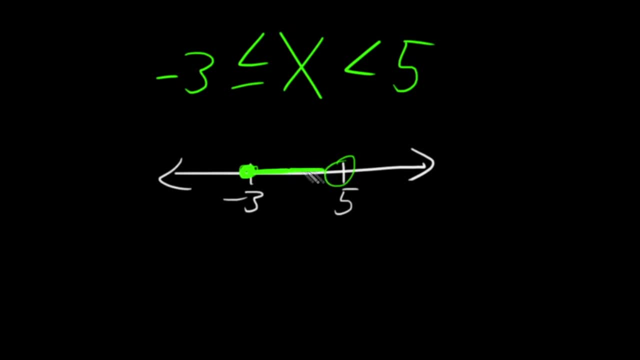 of 5, which looks like this: Let's put down the numbers from left to right. We have negative 3, comma 5, negative 3 was closed circle because it was or equal to That gives us a bracket And then on. 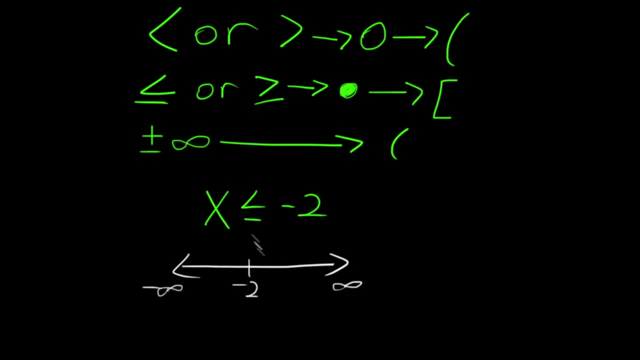 infinities. This time the x is less than or equal to, so we need to use a closed circle to show that we're including the negative 2. And we'll be shading to the left, since it was less than The leftmost amount is negative infinity comma and we're going up to negative 2. Infinities: 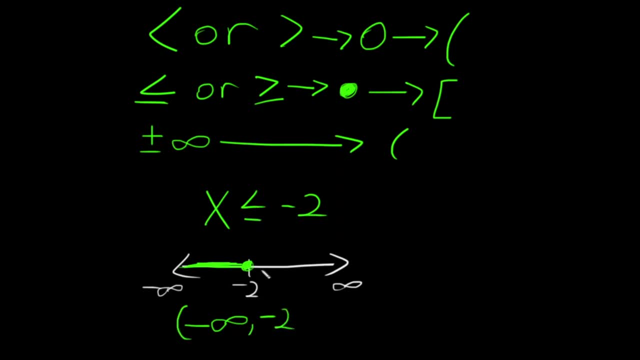 always have parentheses And this time, since we're less than or equal to and we have a closed circle, we're going to use a bracket. Now let's look at compound inequalities. Say, we have x, which is less than or equal to negative 3,, but less than 5.. If we're reading this, inequality left. 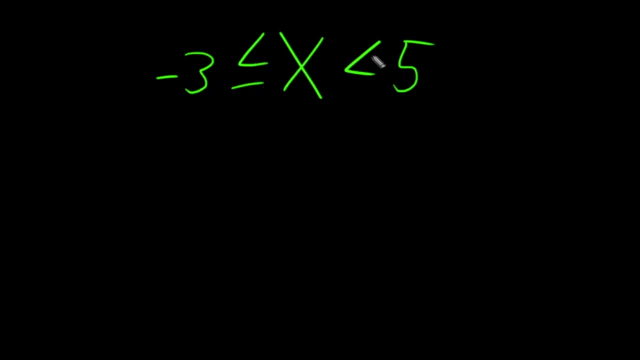 to right. it does say negative: 3 is less than or equal to x, which is less than 5.. But to keep it simple, we can read it starting with the x. In this case x would be greater than or equal to. 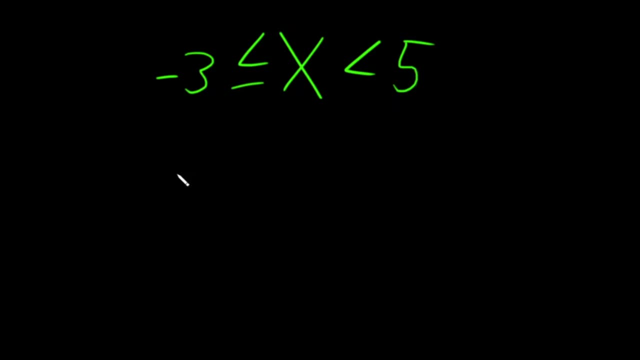 negative 3 and still less than 5.. First let's plot those two numbers on a number line. If negative 3 is over here, then 5 needs to be somewhere to the right over here. First let's do the circles and. 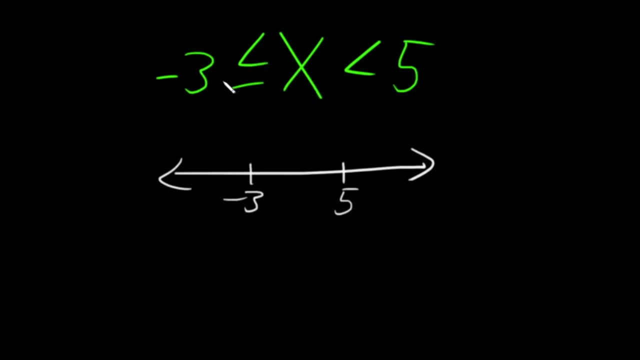 then we'll do the shading. x was greater than or equal to negative 3,, but less than 5.. If we're reading this, then x is greater than or equal to negative 3, so we're going to need a closed circle at negative 3.. On the other side, x is less than 5,, which does not include 5, so therefore we 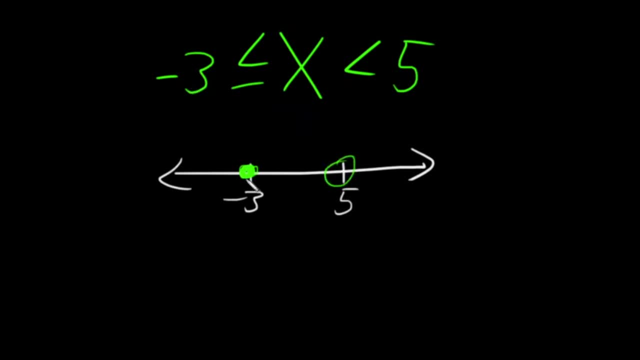 need an open circle. Since x is greater than or equal to the negative 3,, we need to shade to the right from negative 3.. And looking at the 5 side, x is less than 5, so we need to shade to the left. 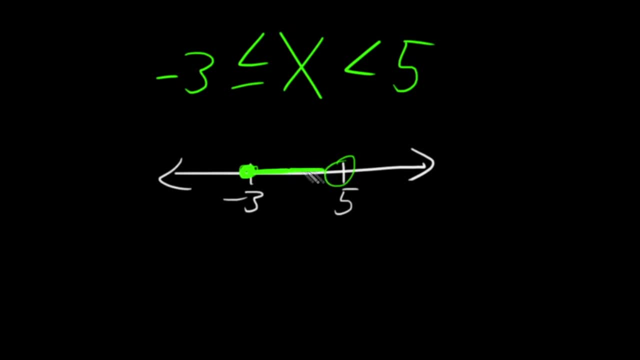 of 5, which looks like this: Let's put down the numbers from left to right. We have negative 3, comma 5, negative 3 was closed circle because it was or equal to That gives us a bracket And then on. 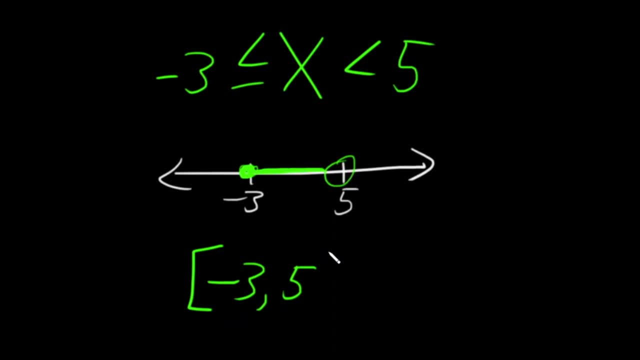 the 5 side. it was just less than and not including the 5,, so we'll just use parentheses. Now, what if we have two inequalities, one where x is less than 0, or x is greater than or equal to 3?? 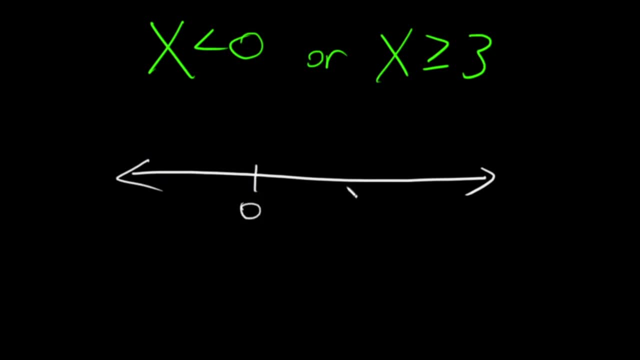 Let's use the number line, Let's plot 0 here and 3 somewhere to the right and use the same rules. First we'll start with the circles. x is less than 0. It does not include 0, so we need an open circle Because it's less than we need to shade. 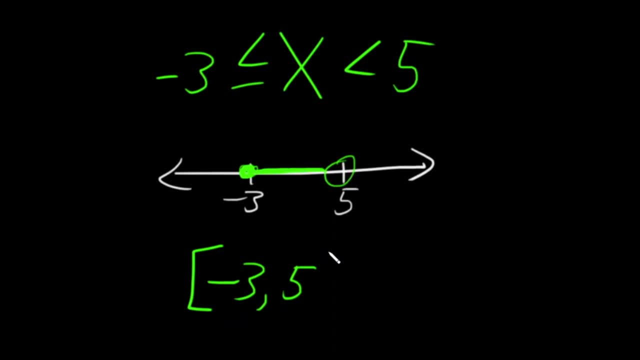 the 5 side. it was just less than and not including the 5, so we'll just use parentheses. Now, what if we have two inequalities, one where x is less than 0, or x is greater than or equal to 3?? 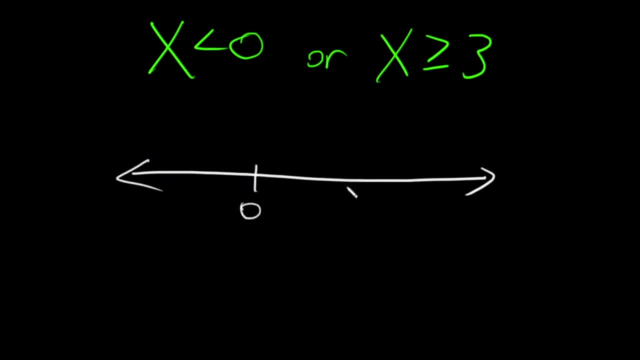 Let's use the number line, Let's plot 0 here and 3 somewhere to the right and use the same rules. First we'll start with the circles. x is less than or equal to negative 4, and therefore included in options. in other words, we include 2 circles. 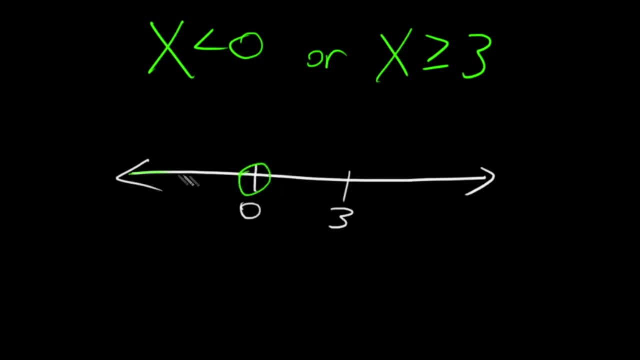 And 1. x is less than 0,, which doesn't include 0, so we use an open circle. Next, x is greater than 1,, which calls for npn 0, and x is greater than 0. We need to shade to the left from 0 to 1.. On the other side, its greater than or equal to 3,. 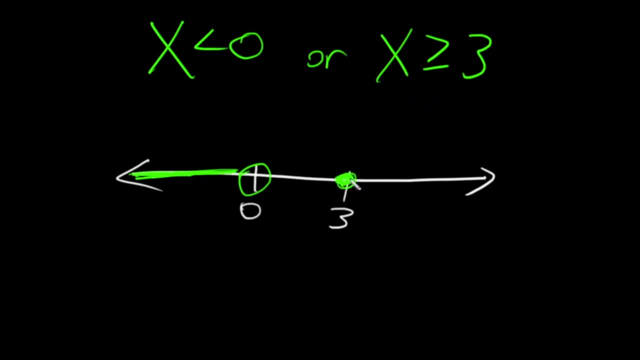 so we include the 3, and therefore include a closed circle. Animal 0 with over 1. BECAUSE x is greater than means 0. Strength chemical energy grill. ultimately, wind factor needs to be from 있으니까. 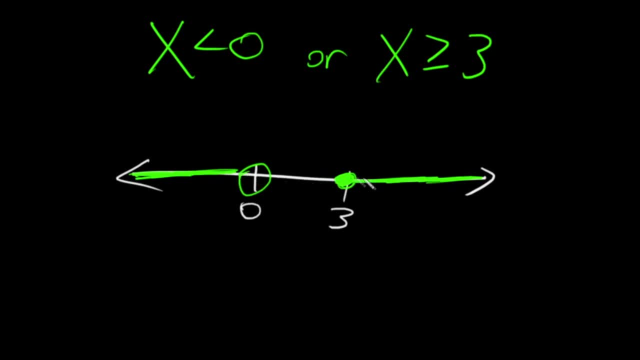 Last time the shadings converged in the middle and this time they're diverging toward the wrong in the overcome events. We know that we're on the right side. we know we're below. we know we're in originals. Right now we're uniformity. 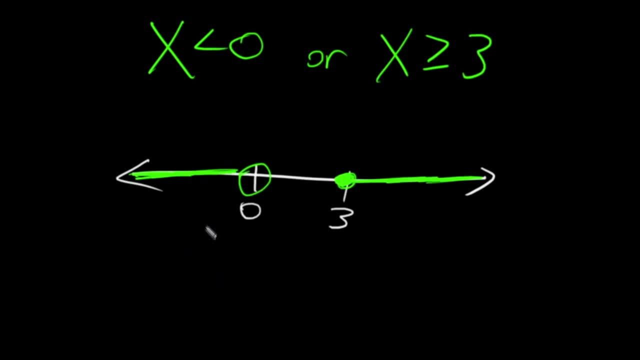 directions. So how do we represent this in interval notation? Let's start with: x is less than 0. We know to the far left is negative infinity, so we're going from negative infinity up to 0. Infinities always have parentheses. This 0 was not included, so we're going to use parentheses On the other. 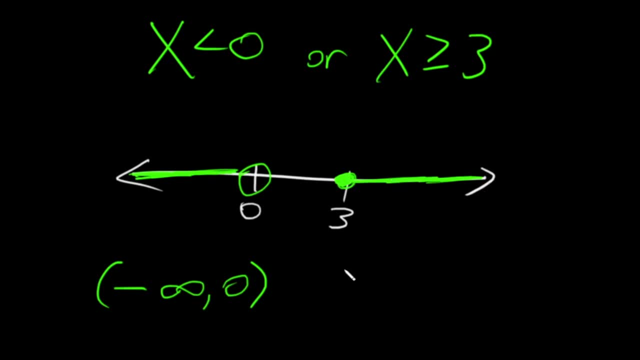 side, we're starting at 3. That's the leftmost of this set, so we need a bracket to show that we're including the 3.. We go from 3 up to positive infinity, close with parentheses, and in between we're going to use a u, which represents union, which joins the two sets together. So, looking at, 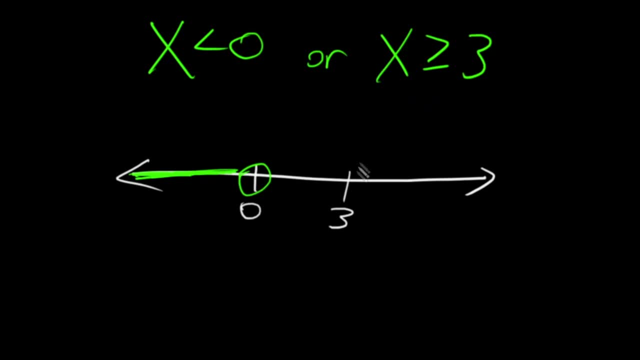 to the left. On the other side, x is greater than or equal to 3,, so it includes the 3, and therefore we need a closed circle And being greater than we need to shade to the right. Last time the shadings converged in the middle and this time they're diverging. They're going. 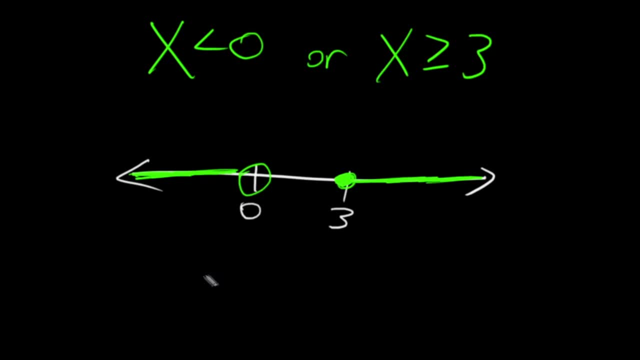 opposite directions. So how do we represent this in interval notation? Let's start with: x is less than 0. We know to the far left is negative infinity, so we're going from negative infinity up to 0. Infinities always have parentheses. This 0 was not included. 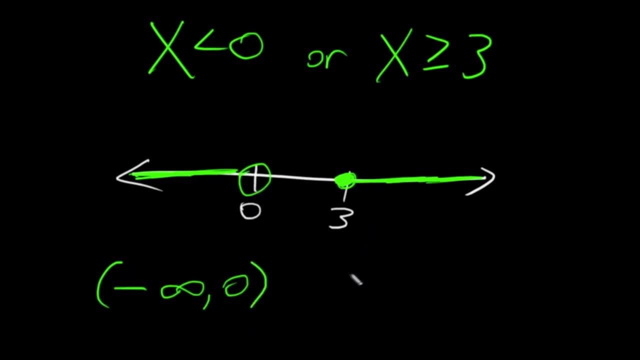 so we're going to use parentheses. On the other side, we're starting at 3.. That's the leftmost of this set, So we need a bracket to show that we're including the 3.. We go from 3 up to positive. 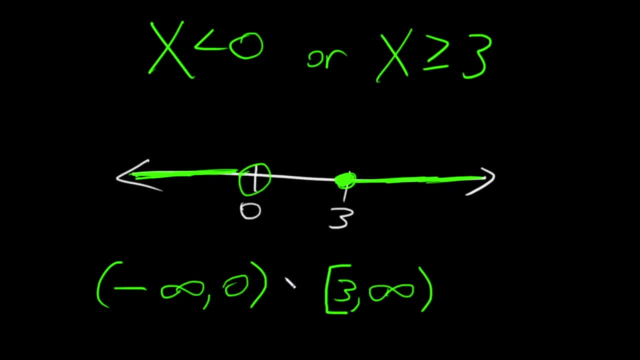 infinity close with parentheses, And in between we're going to use a u, which represents union, which joins the two sets together. So, looking at the notation, we're going from negative infinity up to 0 and stopping without including 0. And then we jump over to 3, including the 3, all the way up. 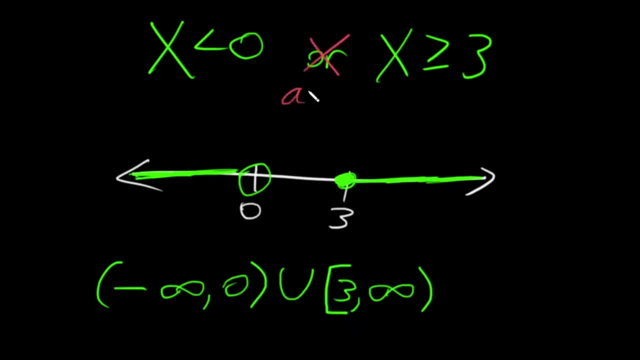 to infinity. Now instead of. or what if this had said: and Is that possible? Let's take a look. Can we have numbers that are less than 0 and also greater than or equal to 3?? Clearly that's not possible, so there's no solution. It would be an empty set Along with the? u representing union. 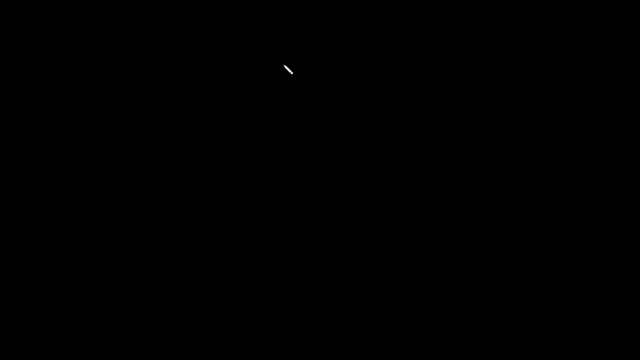 which joins two sets together. there's also intersection, which is represented by an upside down? u like this: Think of the intersection as the overlap between the two sets. For example, let's say x is greater than 1 and x is less than or equal to 6.. To help visualize this, 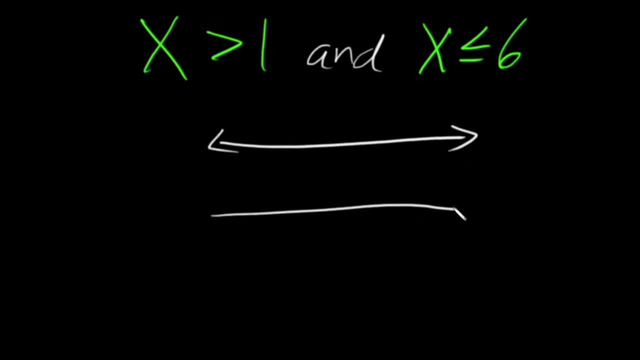 let's draw two number lines, one just above the other. Let's start with: x is greater than 1.. We'll have 1 here. We know we're greater than not or equal to, so we need an open circle, And because it's greater than we'll shade to the right. 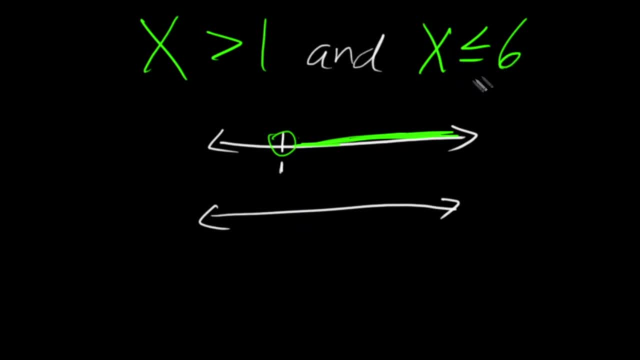 On the other number line we'll graph x is less than or equal to 6. And the idea of having the two number lines is to have them overlapping, as if the numbers lined up. So if 1 is over here for the top number line, then it's directly below on the second number line, meaning 6 is going. 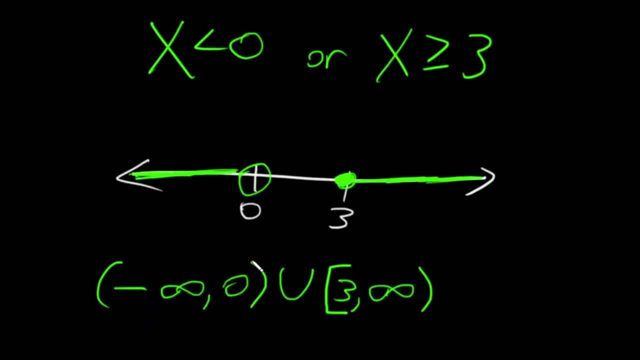 the notation. we're going from negative infinity up to 0 and stopping without including 0, and then we jump over to 3,, including the 3,, all the way up to infinity. Now, instead of, or what if this had said, and Is that possible? Let's take a look. Can we have numbers that are less than 0 and also? 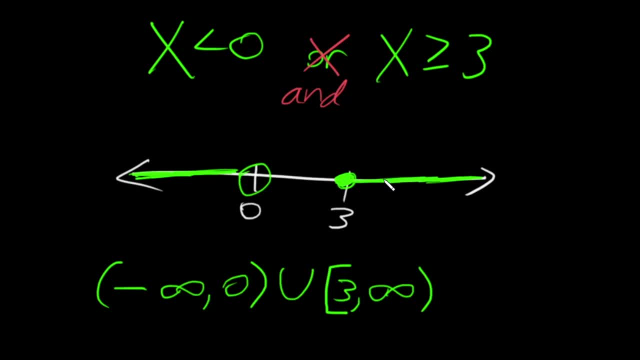 greater than or equal to 3?? Clearly that's not possible, so there's no solution. It would be an mx. So we're going to use an empty set, Along with the? u representing union, which joins two sets together. there's also intersection, which is represented by an upside down. u like this.